gives us a value of 1.5.. Now let's apply our matrix to our basis vectors. We can see that adding the lasting speed to our matrix gives us a value of 1.5.. Now let's add this v after it was transformed by: 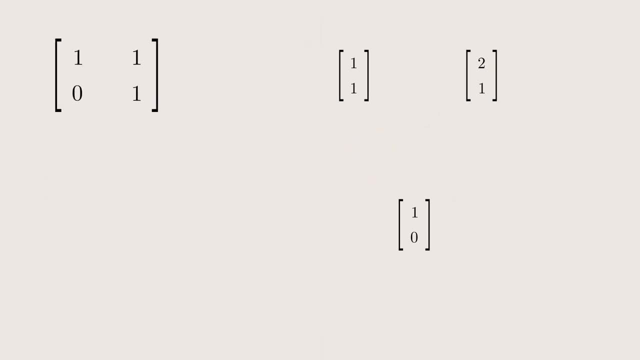 the matrix. On top of that, note that the columns of the matrix are just the transformed basis vectors. Now, since t is also linear, to figure out what it does to v we similarly only need to see what t does to the basis vectors. Furthermore, this process shows us how we could write t. 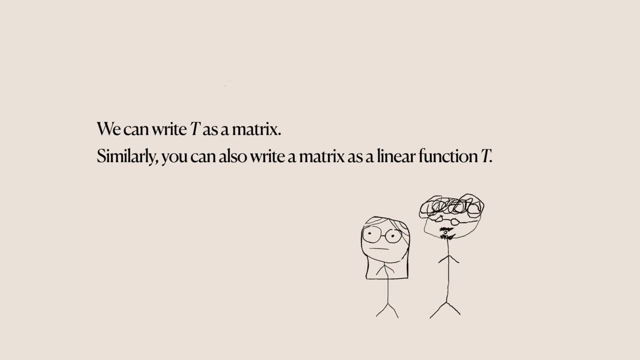 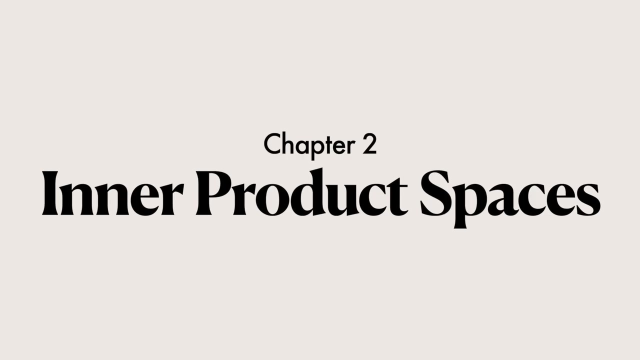 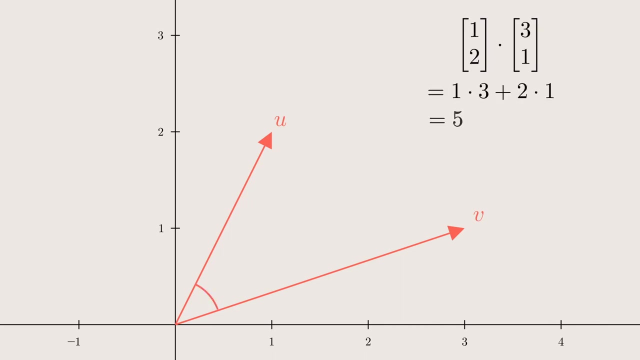 as a matrix. We could also go the other way, starting with the matrix and define a linear function. These special linear functions are called linear operators and there's an exact correspondence between them and matrices. Recall the traditional dot product of vectors When the dot product of two of them is zero. we know that there are right angles. 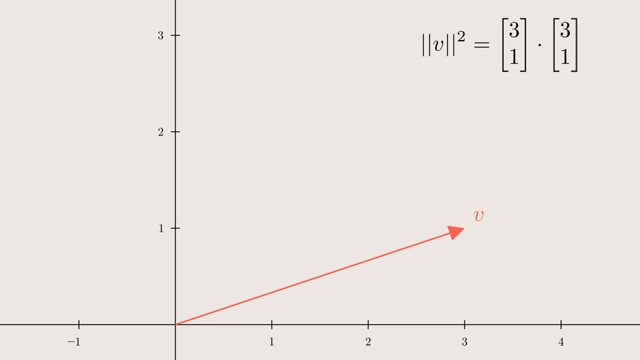 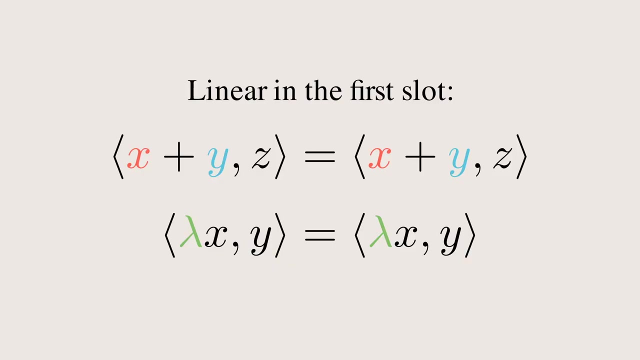 and we can figure out how long a vector is by taking the square root of the dot product with itself. We can generalize the concept of the dot product to an inner product. This is a function on a vector space which is linear in the first component. 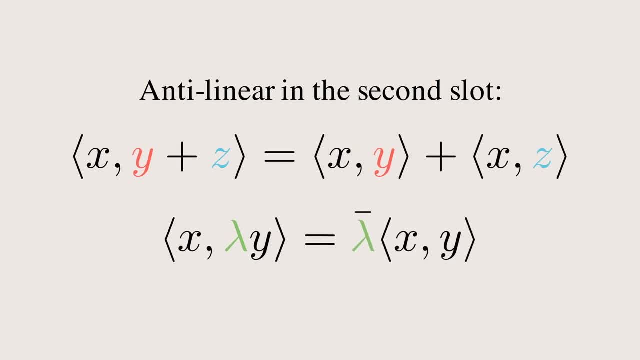 it's conjugate, linear in the second component and it's non-negative, only giving zero. if what you plug in is zero, We can then use the inner product to define a norm, just as we did with the dot product, the square root of a vector. inner product with itself. 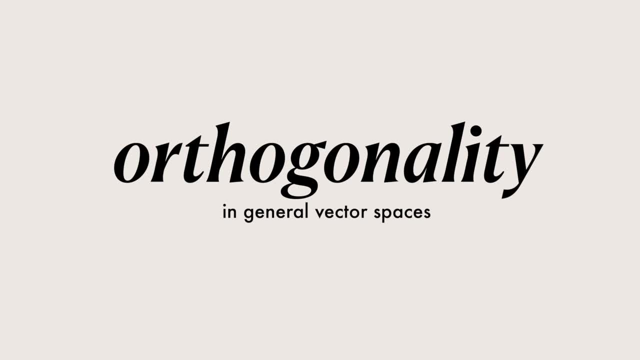 Inner products. also, let us define orthogonality and arbitrary vector spaces. We say two vectors are orthogonal if their inner product is zero, which just generalizes the concept of right angles. We can also define one of the terms we saw at the beginning, the adjoint Given a linear operator t, it's a. 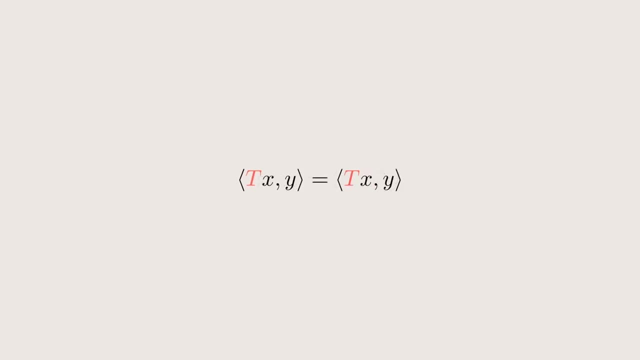 joint key. star is the unique linear map, so that tx inner product with y is equal to x inner product with t. star y for all vectors x and y. If we choose to represent our linear operator as a matrix, the adjoint is given by conjugate transposition. 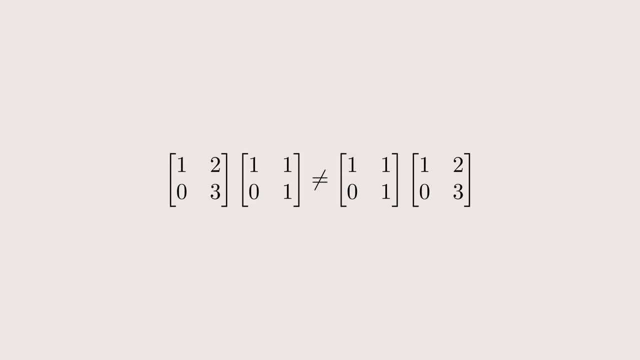 We know that not all matrices commute and we know matrices are just linear operators in disguise. so not all linear operators commute either. If t commutes with its adjoint t, the vector space is defined as the unit vector of v, which is the unit vector of v. We can do the same thing with the. 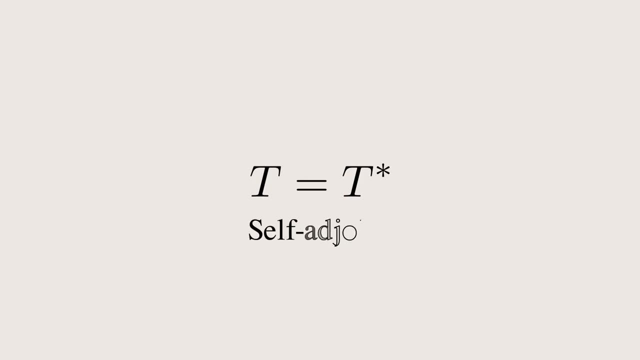 dash line t star, that we call it normal. If t and t star are the same operator, we say t is the adjoint. Consider the red unit vector v, where the dash line is its span. Now draw any other vector u. We can find two vectors, one of which lies on the span of v, the blue vector. and then we can find the other vector, u, which is the unit vector of v, which is the unit vector of v. 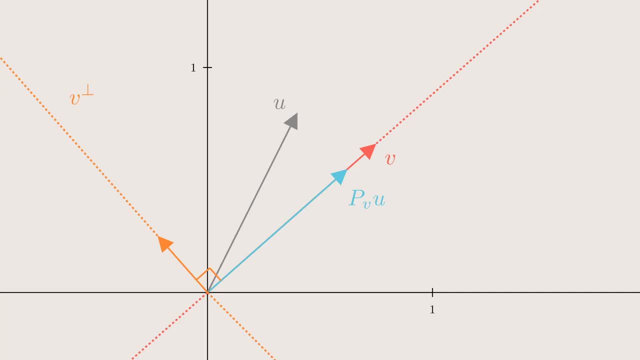 In this orange vector that lies in the orthogonal complement or the set of all vectors that are orthogonal to V. when we add the blue and orange vector together, we get U. This is how we define vector projection, because these choices are unique and so we call the 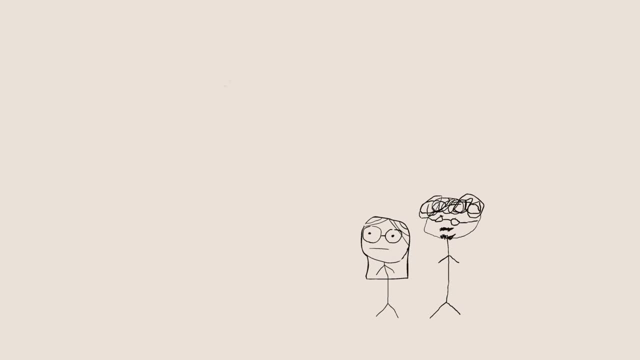 blue vector, the projection of U onto V. We can now combine everything we've learned into one big theorem, the spectral theorem. It tells us that if we have a normal operator over a complex vector space or a self-adjoint theorem, if we have a real vector space, then its eigenvectors form an orthonormal basis. 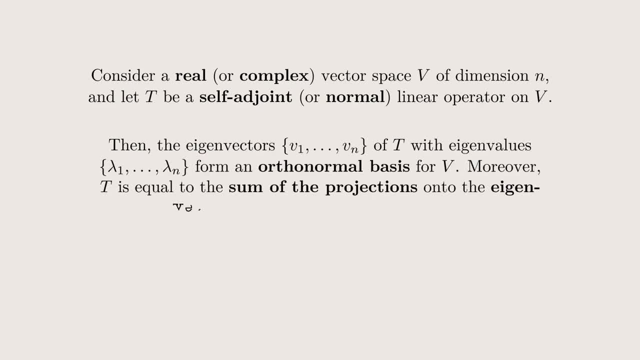 for the space. On top of that, we can write the operator as the sum of projections onto these eigenvectors, weighted by their eigenvalues. Okay, but what does this actually mean? Consider the following real self-adjoint matrix and: 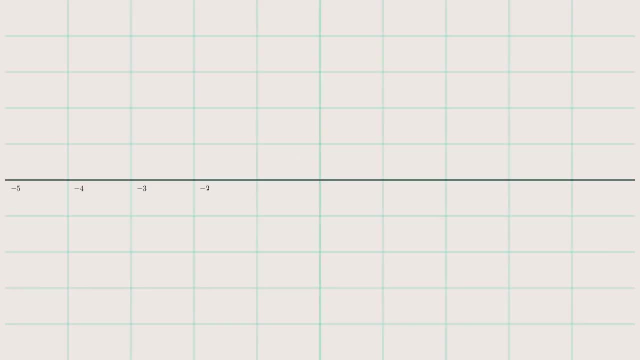 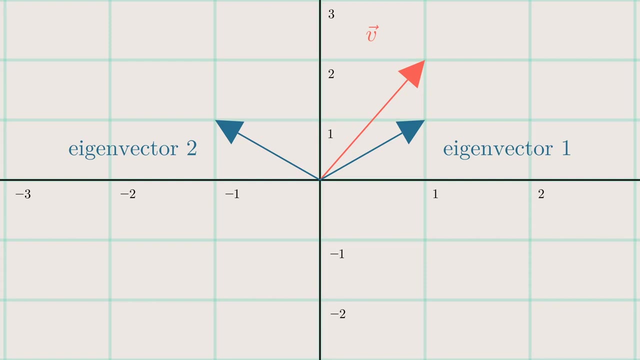 note that since it's real, this really just means it's symmetric. Its eigenvectors are written in blue and we know that by the spectral theorem they form a basis for our space. Can we figure out what our matrix does to our red vector V in terms of what it does? 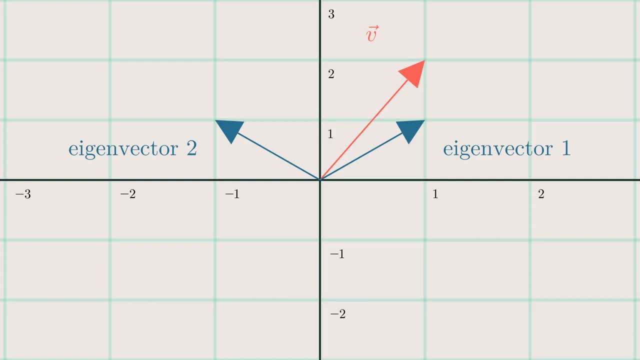 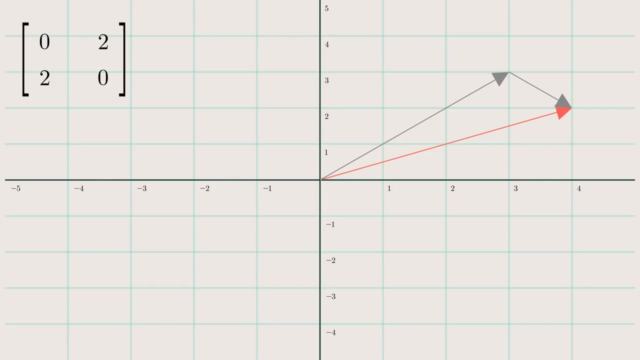 to these eigenvectors. Well, yes, If we project V down onto each eigenvector, scale it by the eigenvalue and then sum up the result, we'll end up getting what the matrix does to V. It's really just a bunch of simple vector projections in disguise. 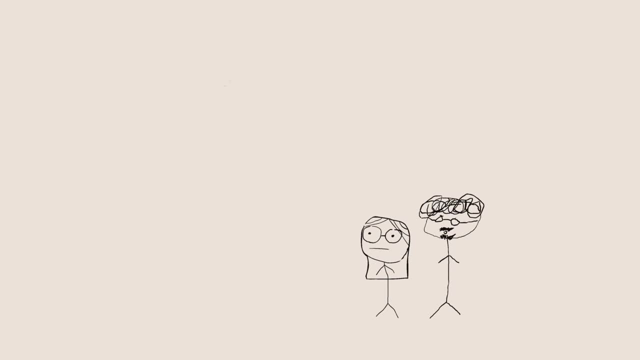 These matrices and linear operators- normal and self-adjoint ones- really are a special class. however, If you just pick a random matrix or a random linear operator and you do this down, projecting onto its eigenvectors and scaling, you might end up nowhere close. 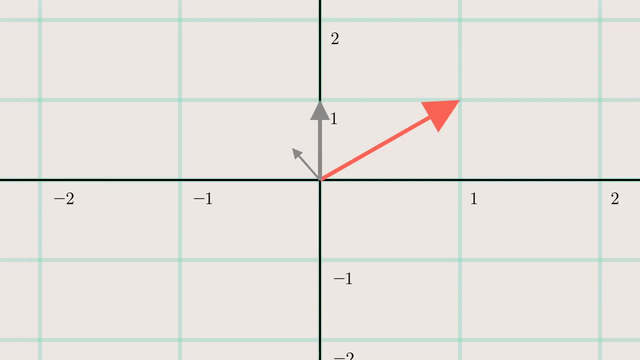 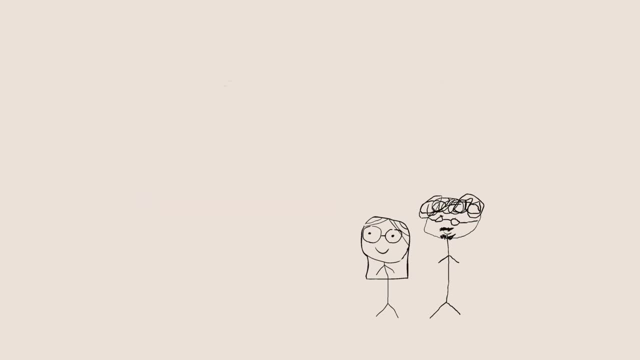 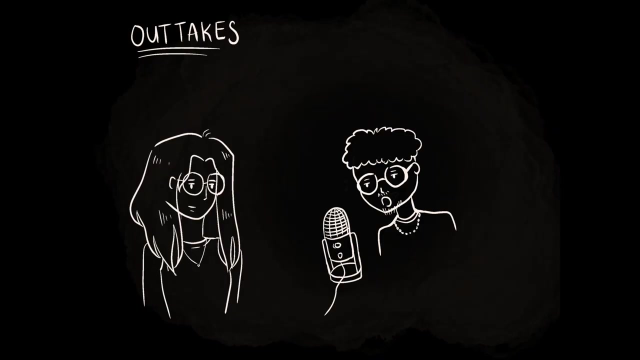 to where you're supposed to be, so just be careful. I'm eating ham To describe this thing. 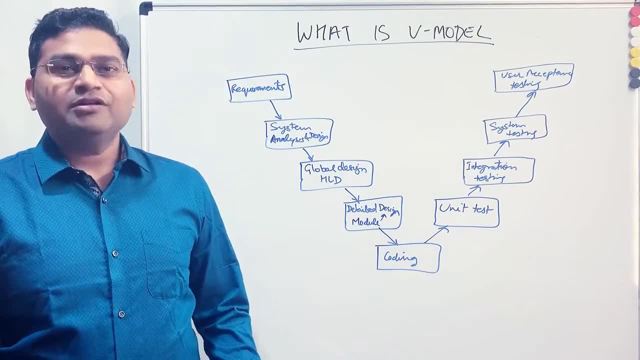 Hello everyone, Welcome again. In this software testing tutorial we are going to learn what is vModel. So we have already understood about the waterfall model in the previous tutorial of a software development lifecycle. So there is a waterfall model that teams used to follow. 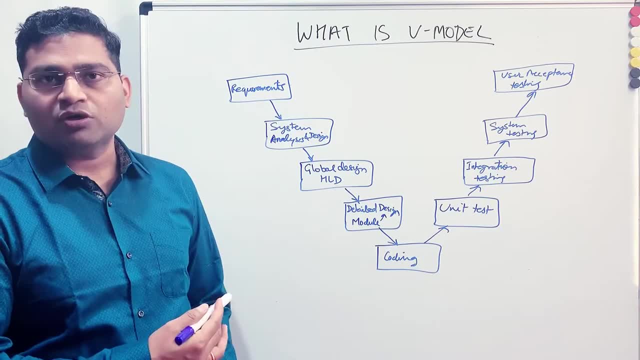 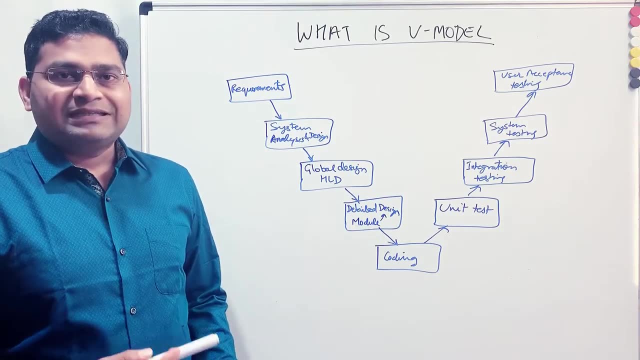 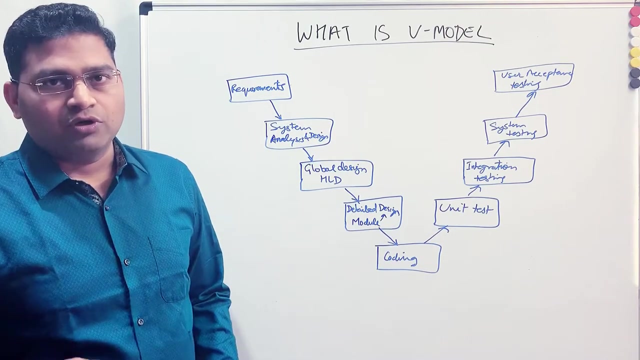 and because of the disadvantages that we have discussed in the waterfall model, vModel got involved. So the major disadvantage in the waterfall model was around the delay in the feedback right Or the testing phase was delayed a lot in that particular waterfall approach. 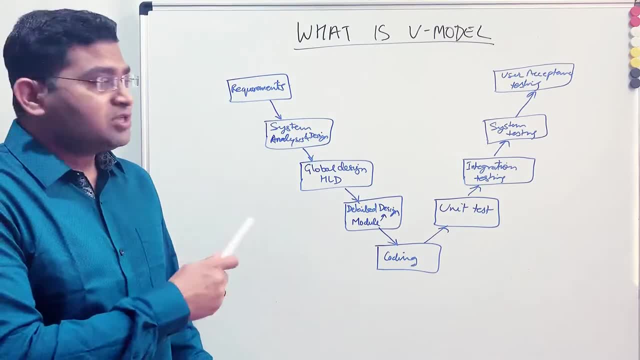 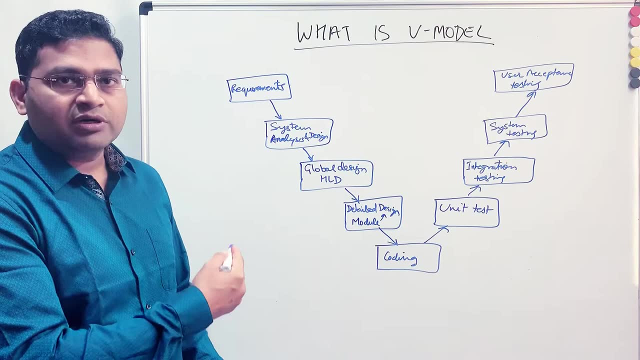 So if you haven't watched the previous tutorial, please go ahead and watch it first before you come to the vModel, because both of them are interrelated and vModel is an improvement over the issues that were there in the waterfall model, So you need to understand the waterfall model. 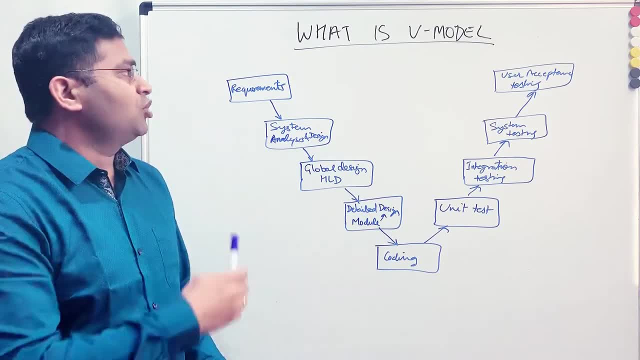 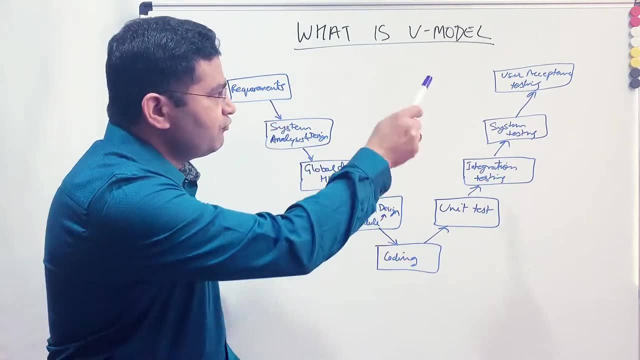 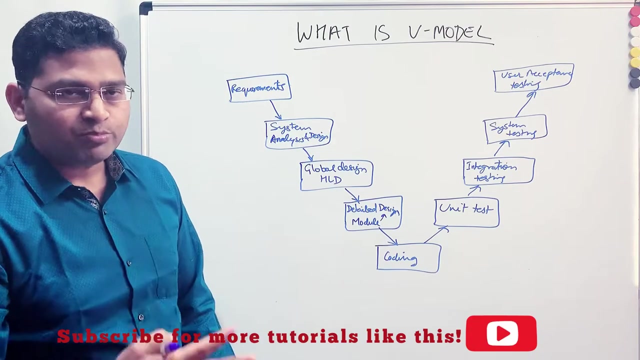 first before you Are able to understand what vModel is. So, as you can see on my screen, the vModel, as the name suggests, it's in the shape of V, rather than the waterfall approach wherein all the phases were one after the other. vModel is a bit of an improvement, even though there 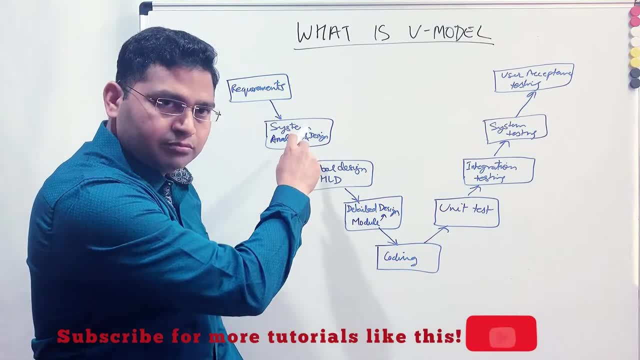 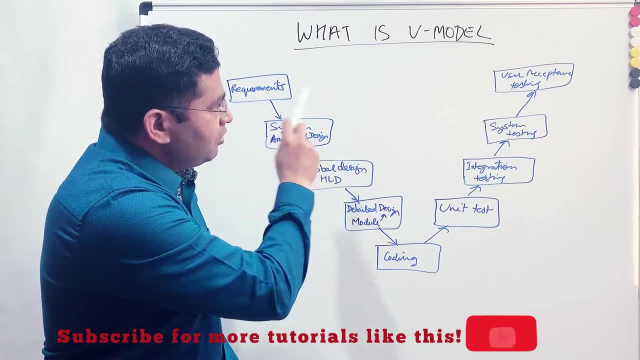 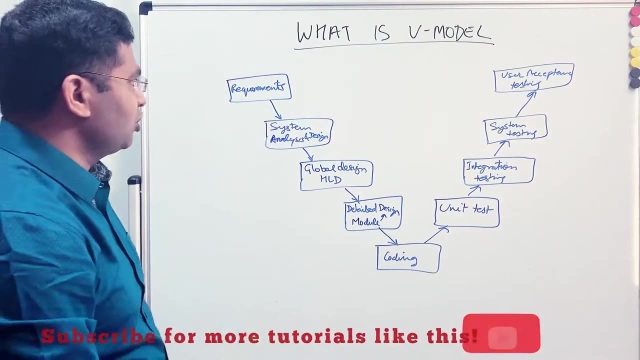 is still the phased approach and there are, you know, phases after the other, one after the other, but still there are corresponding phases of testing for each of them: The development phase or the requirement phase. So let's understand what exactly vModel.